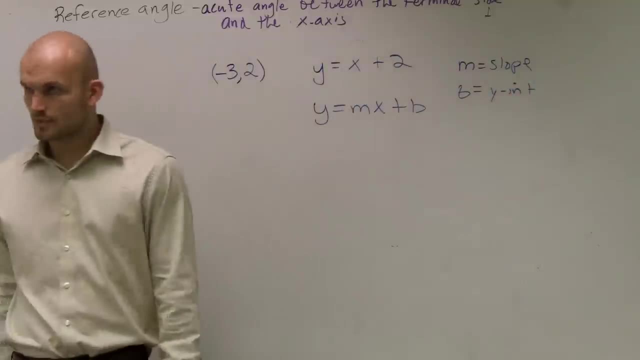 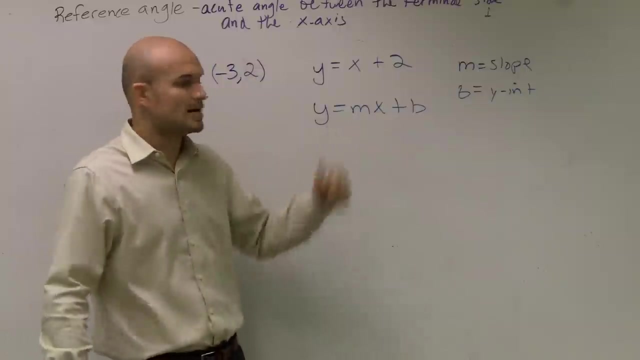 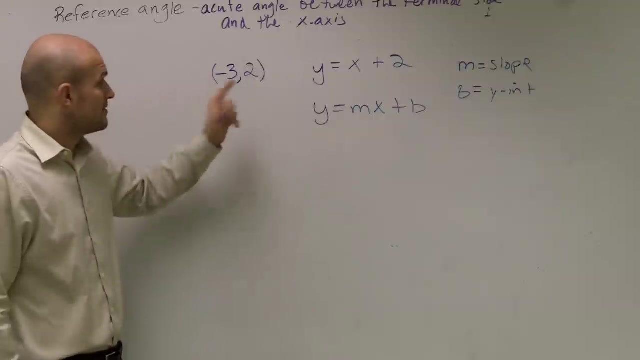 our y-intercept right. So my problem, that's probably the first information I can write down. All right, I know our equation. I can write down: y equals mx plus b, all right, Now the next thing is it says: find a perpendicular line that goes through this point. that's perpendicular, Sorry. 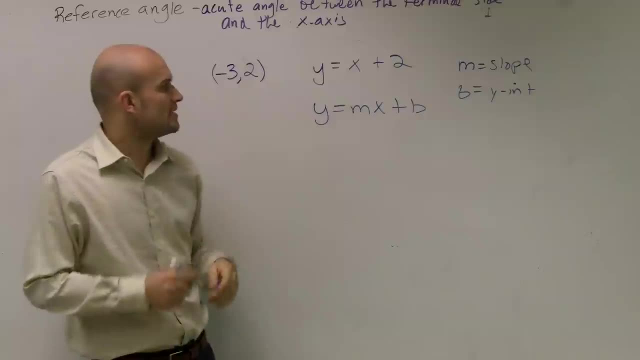 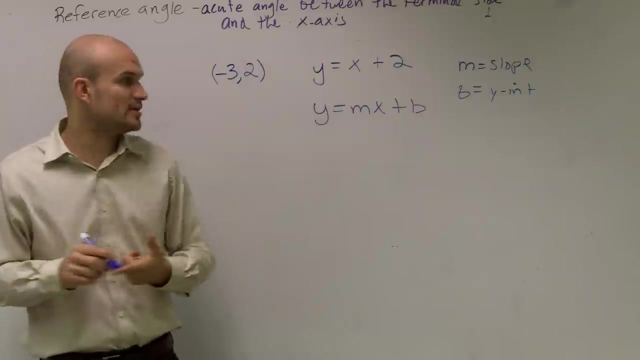 find a line, A line that goes through negative 3,, 2, but that goes through, that is perpendicular to y equals x plus 2.. So what we need to do is we need to say: all right, with that information, can we figure? 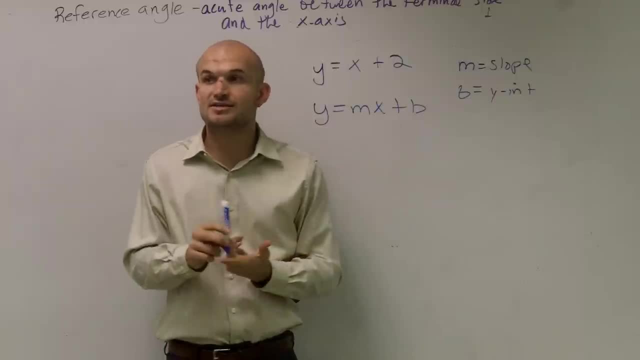 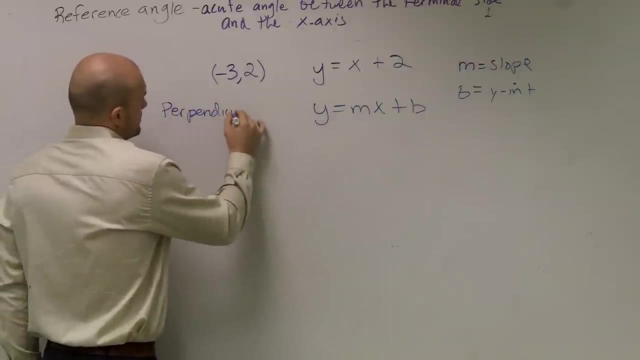 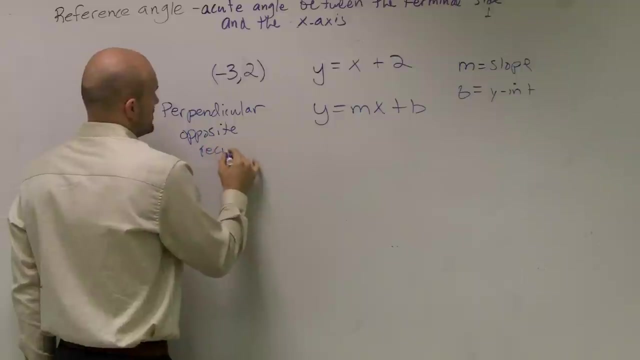 out what the slope and the y-intercept is. Well, the first thing, guys, is we can remember, we can figure out the slope, because one thing about perpendicular lines: perpendicular lines have what we call opposite. So what that means is, if I have my slope over here, let's say I'm giving a ramp slope of 1- 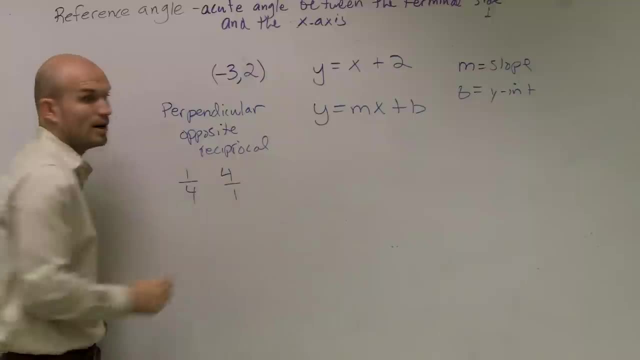 fourth, the reciprocal is 4 over 1.. And remember, the opposite means if one is positive, then the other slope is negative. So those are what we call opposite reciprocal slopes. So what here I need to look at and say: well, what is the slope for? y equals x plus 2? And this 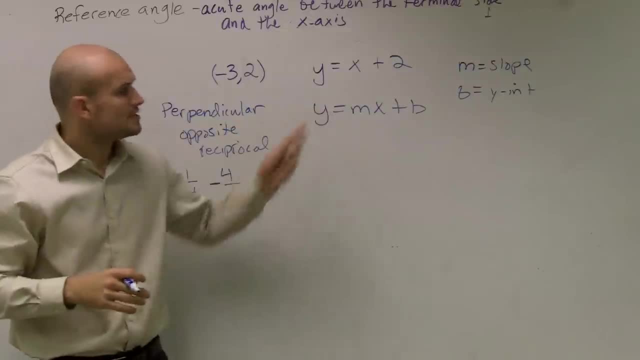 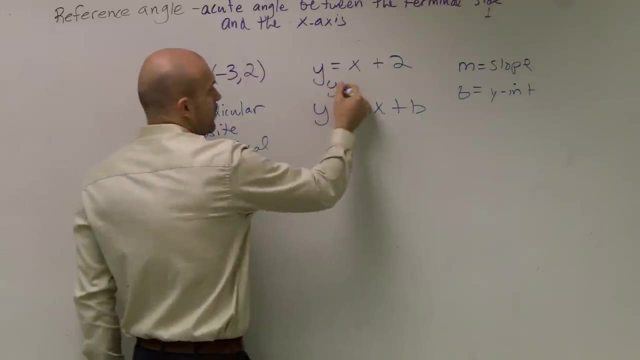 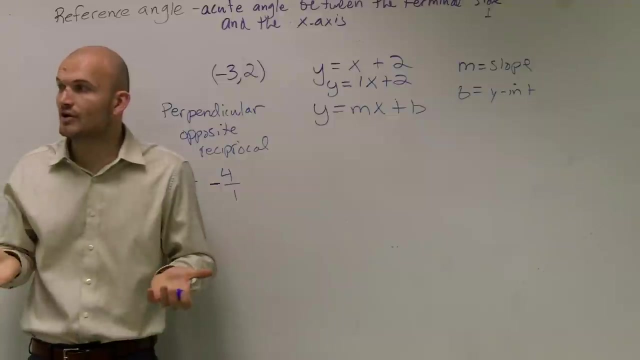 problem is difficult. This problem is difficult because, I don't know. there's no number in front of the x. Well, we need to remember that y equals 1 over x plus 2, right, If there's no number in front of our x, we can assume that 1 is in front of there, because 1 times. 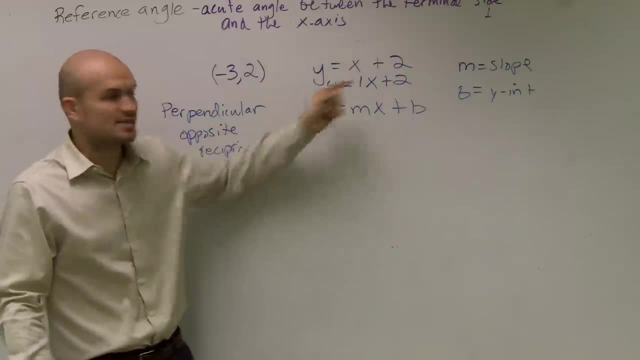 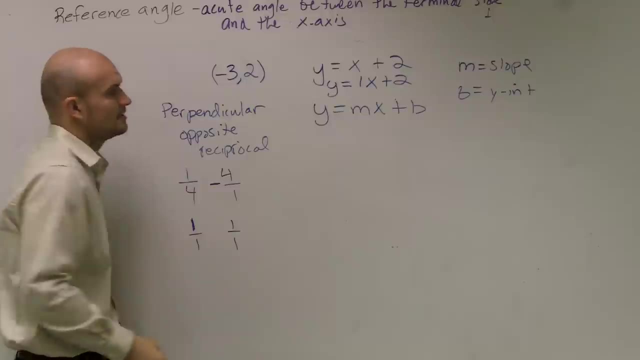 x is going to give you x. So I need to look at what is the reciprocal of 1?? And you could say: well, the reciprocal of 1 over 1 is 1 over 1.. And since this is positive, to make it opposite, it's going. 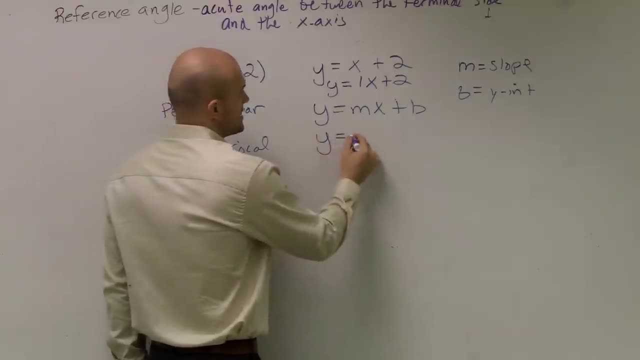 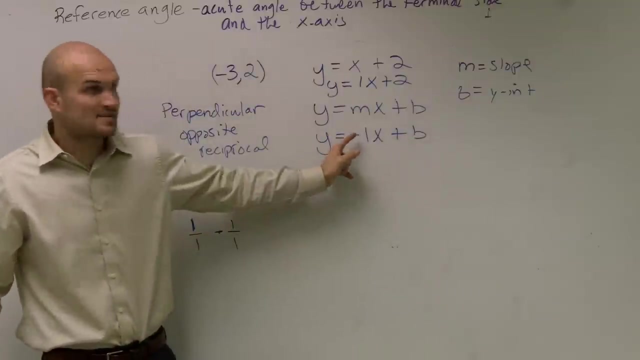 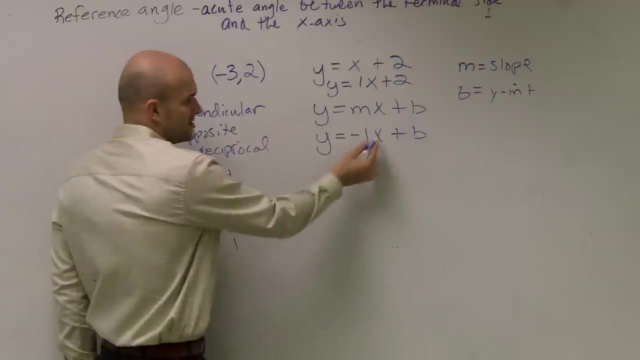 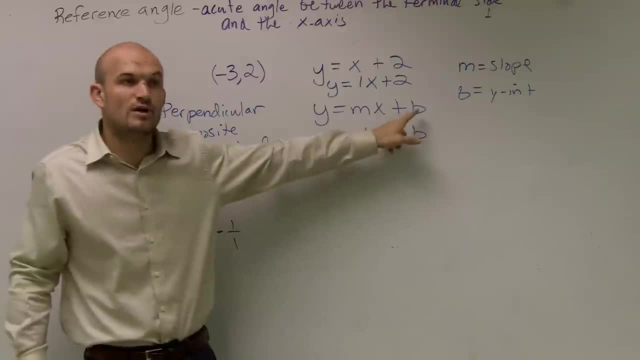 to have to do this. I'm going to have to do this. I'm going to have to do this. Now. we've got y equals mx plus b. We've figured out what the slope is. Now we need to figure out what our y-intercept is. We still don't know what the y-intercept is, The biggest. 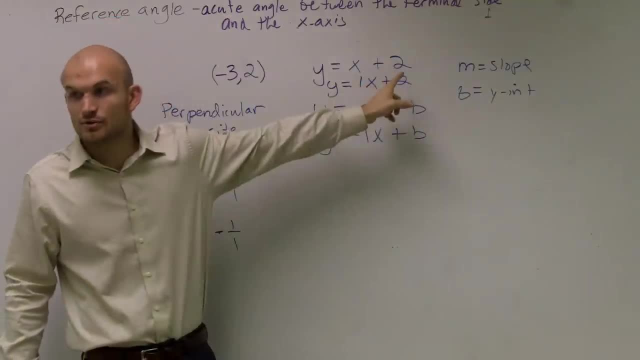 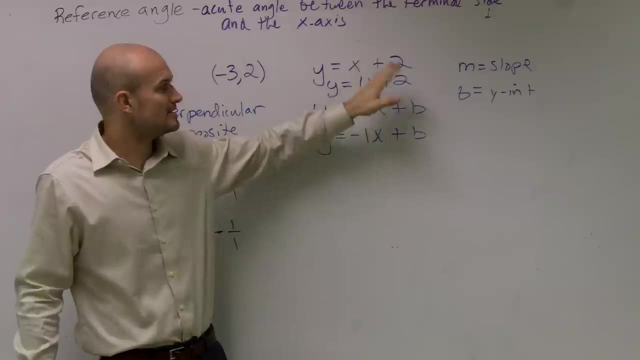 mistake that students want to do is they want to say your y-intercept is 2.. Well, for this equation your y-intercept is 2. But for a line perpendicular to 2, it's not going to be the same y-intercept. It could be, but let's go and determine if it is Yes. 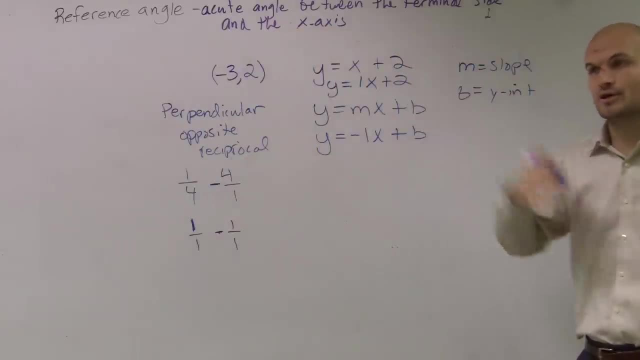 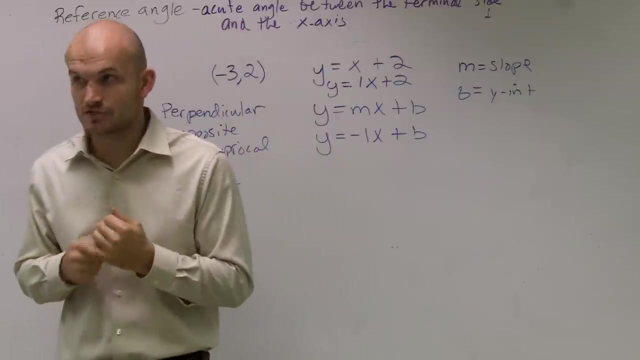 Why do we have to be the 2 hashtag? Well, let me go and show you, Let me go and see, Let's go and determine if it is or not Happy birthday to you. Happy birthday to you or not? because, before it can be, the y-intercept of 2,. 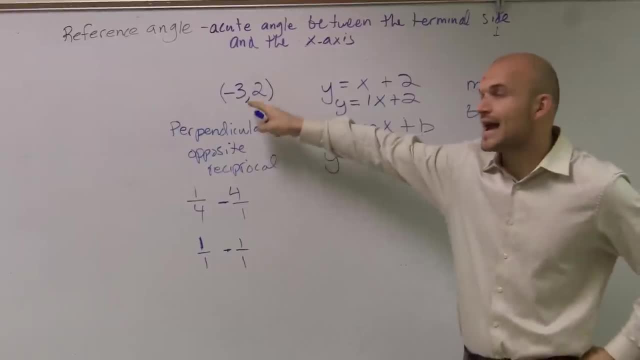 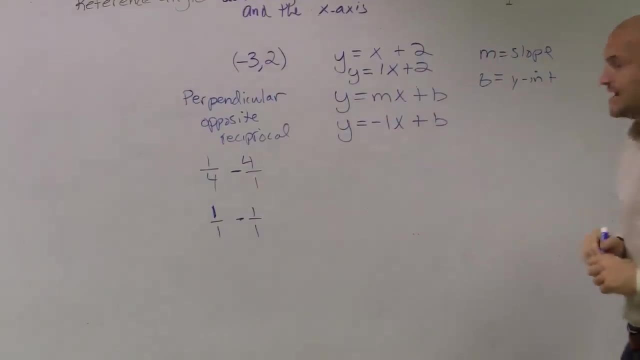 we have to see. there's one thing it says. It says the graph has to go through negative 3 and 2.. So therefore my graph has to go between negative 3 and 2.. So to do that, I can say: well, every point. 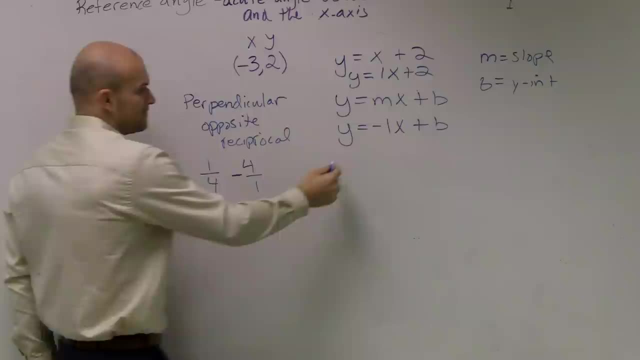 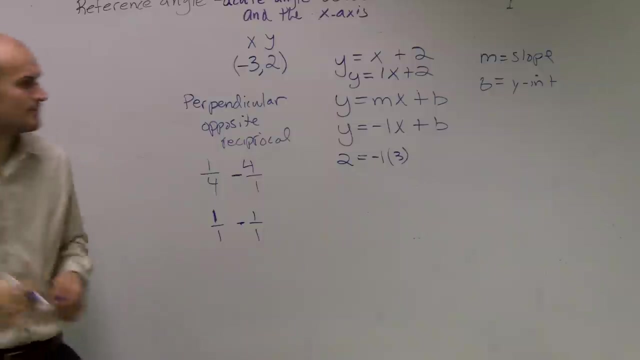 has an x and a y-coordinate, So I'll plug in 2 and for y and 3 and for x. John, can you be cognizant? Negative 3,- thank you, Plus b, So therefore I do a negative 3 times negative 1. 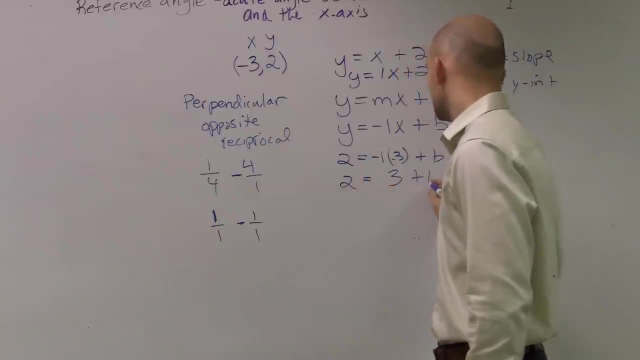 is going to give me a positive. 3 equals 2 plus b. Now when I solve for b, I'm going to subtract the 3, and I actually get a y-intercept of negative 1.. Do you guys see why my y-intercept is negative 1? 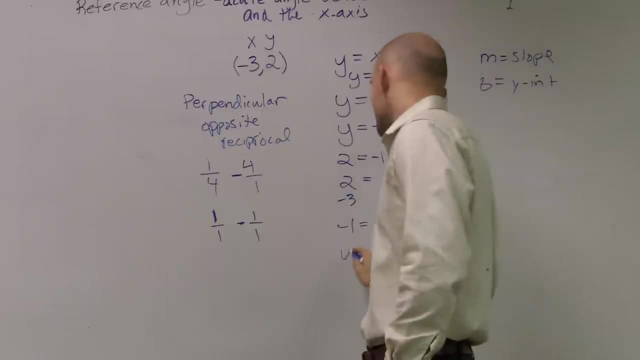 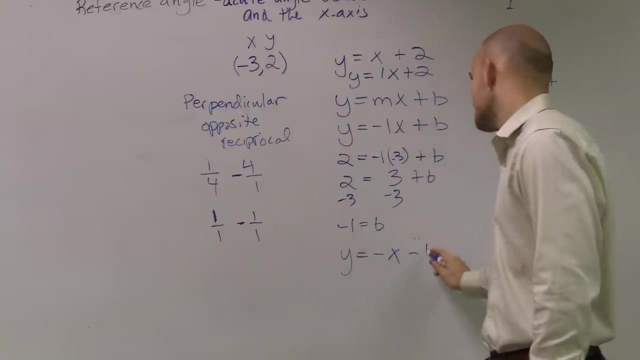 and it's not 2?. So therefore, my final line, My final equation, is: y equals my slope, which is a negative 1 times x minus 1.. So y equals a negative x minus 1.. Or, if you wanted to write it in the slope-intercept: 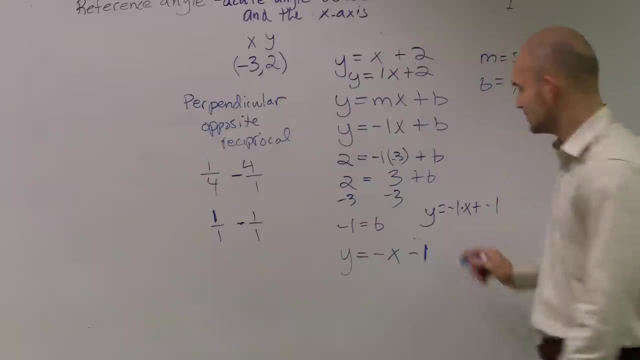 y equals negative 1 times x plus a negative 1.. But the simplified version. Any questions on that? The main important thing, guys, about perpendicular lines: you have to understand perpendicular lines have the opposite and reciprocal slope, If you can remember opposite and reciprocal slopes.